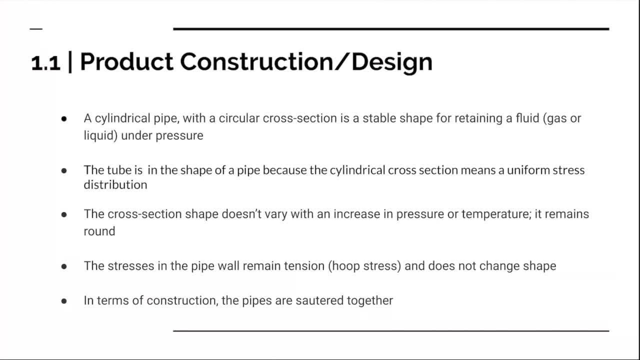 is a stable shape for retaining a fluid, whether it's a gas or liquid, under pressure. A cross-section shape doesn't vary with an increase in pressure or temperature. It remains round, The stresses in the pipe wall, remain tension- ie the hoop stress- and does not change shape at all If the 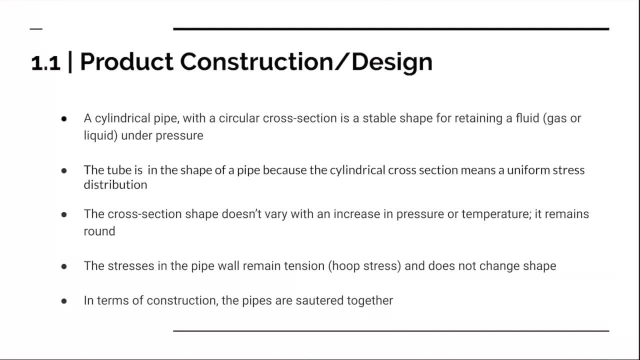 pipe's cross-section were elliptical, though, and an internal pressure would try to make the cross-section round, Increasing the stress and decreasing the fatigue strength. Also, the pipe hangers of mounting would be abnormally loaded and could fail. And then, in terms of the construction, the pipes are all when they come. 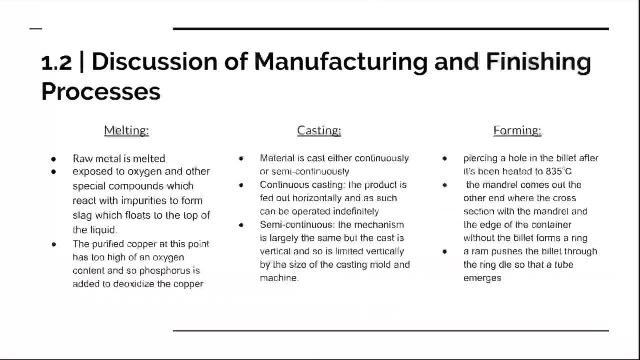 to being put together. they are all soldered together. Next up, we're going to be talking about the discussion of manufacturing and finishing processes, And the material we have chosen is the copper piping. Copper pipes for plumbing are made of nearly pure copper, with some 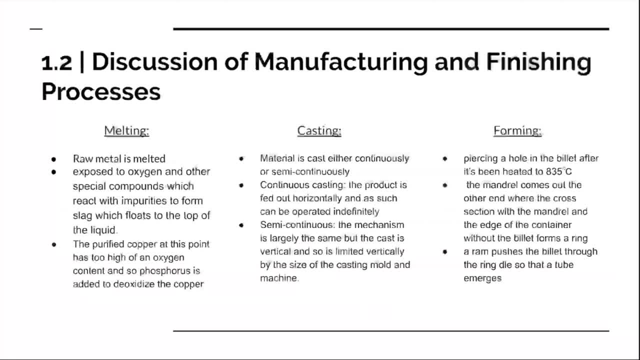 silver impurities and phosphorus. So first thing is melting. Well, raw material is first melted. This is the first step in purifying the metal. The temperature is usually between anywhere from 1,200 to 1,400 degrees Celsius. It 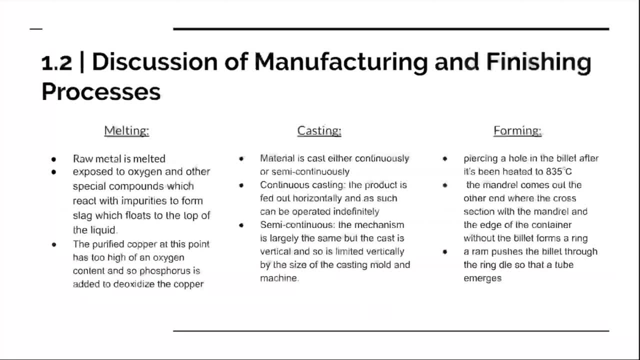 is then exposed to oxygen and other special compounds which react with impurities to form slag which floats to the top of the liquid. The purified copper at this point has too high of an oxygen content and therefore phosphorus is added to deoxidize the copper. Now it is prepared for. 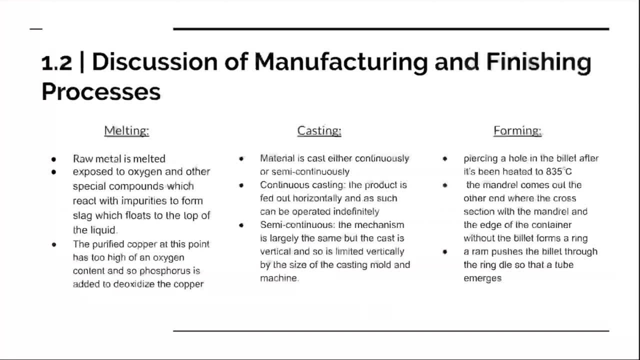 casting. The second step is casting, where the material is casted into a copper pipe. The copper is casted to a copper tube that flows through a battery, which is then removed from the copper pipe at the moment of casting. This is where the copper is casted and then the copper is added by the copper tube. 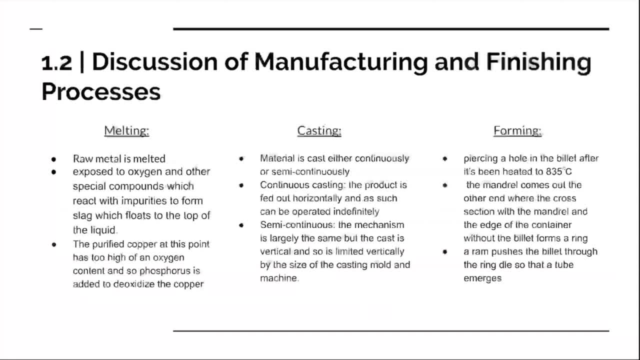 is casted to the copper tube. The first step is melting. This is the first step in cast either continuously or semi-continuously. In both casting processes, the melted material is poured at a controlled rate. The walls of the mold are cooled, causing the copper to solidify. 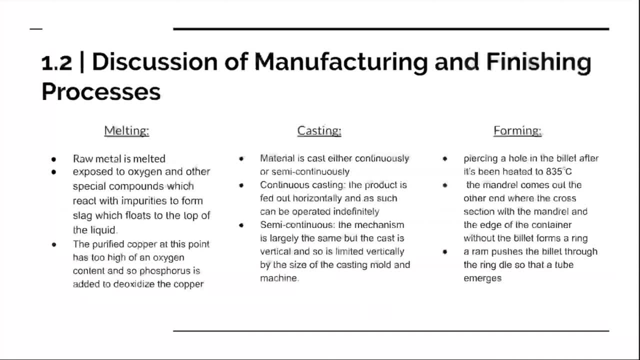 In continuous casting the product is fed out of horizontally and as such can be operated indefinitely, While in semi-continuous the mechanism is largely the same, but the cast is vertical and so is limited vertically by the size of the casting mold and machine As such. 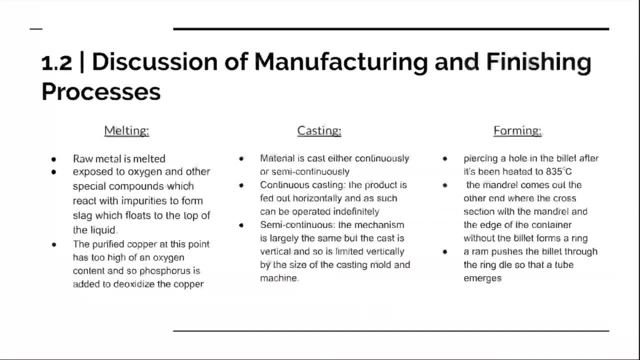 it is going to be halted periodically to make room for casting to continue. Now, the cast is a huge heavy cylinder of copper which is cut into billets. The billets are what are used when forming. The third step in forming involves piercing a hole in the billet after it's been. 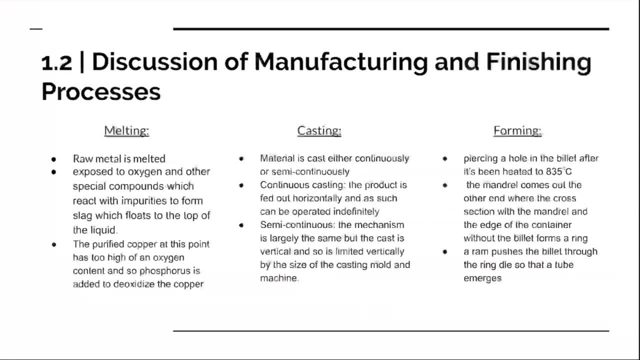 heated to approximately 835 degrees Celsius. A piercing mandrel is driven through the material to create a center hole- the eventual ID of the pipe- and is pushed through the whole billet. After the billet is pierced from one end, the mandrel comes out the other end, where the cross. 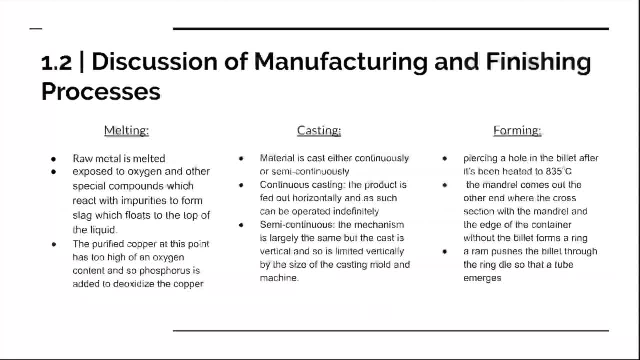 section with the mandrel and the edge of the container without the billet forms a ring. Then a ram pushes the billet through the ring die so that a tube emerges From there. the tube is put through a process called drawing, where it moves through a variety of dies so that the tube is in. 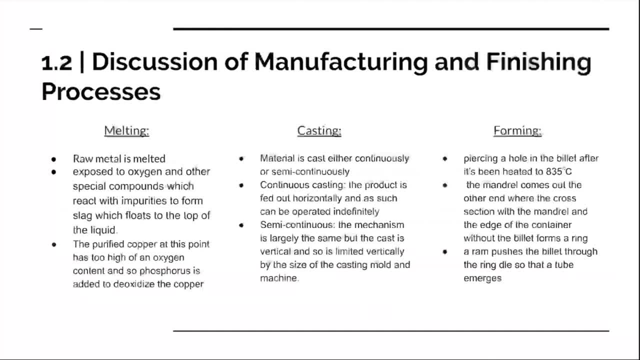 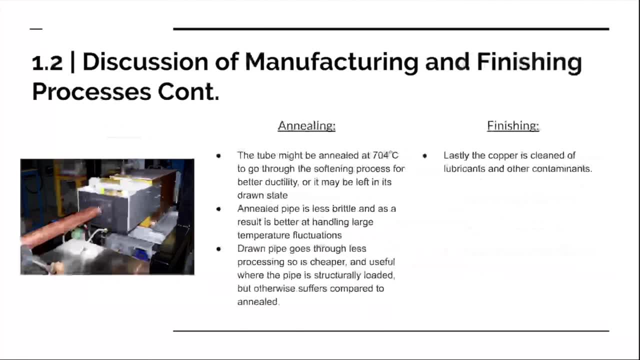 the correct dimensions. This strain hardens the material, so it comes out quite strong. Next up we have annealing which, depending on the desired properties, the tube might be annealed at 704 degrees centigrade to go through the softening process for better ductility, or it may even be. 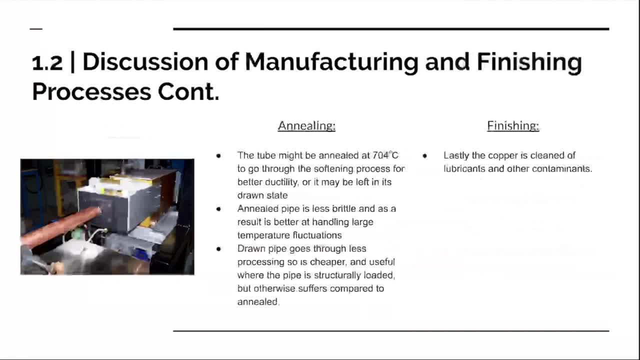 left in its drawn state. An annealed pipe is less brittle and, as a result, is better at handling large temperature fluctuations. It can withstand higher pressures without failure but might deform, leading to failure, and can be bent, which is useful for some applications. Drawn pipe goes through less processing, so it's cheaper. 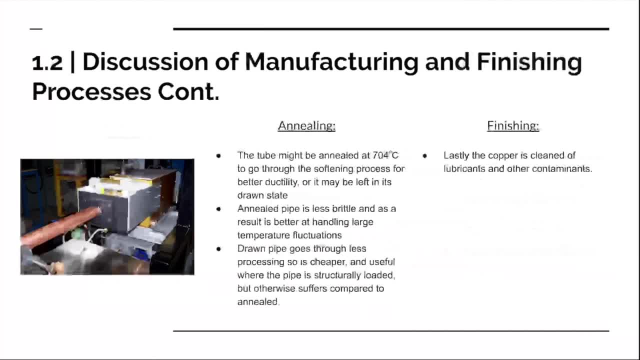 and is useful where the pipe is structurally loaded but otherwise suffers compared to being annealed. And then the last finishing touches is that the copper is cleaned of lubricants and other contaminants. This is especially important for plumbing lines, as the water needs to be potable. 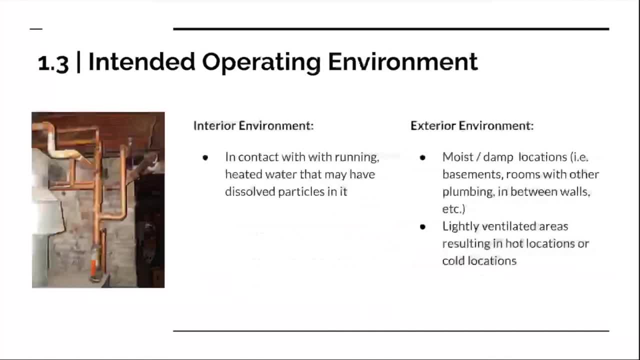 going into something like a tap. In terms of what the intended operating environment for the tube is, well, we have an interior and exterior. In interior, the copper pipe itself will be in contact with running heated water all the time that may have dissolved particles in it, While the exterior environment usually the heaters 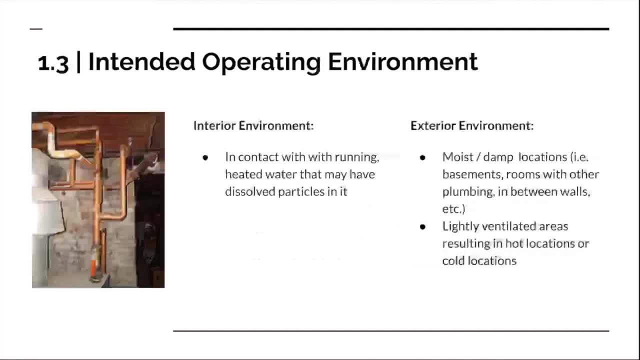 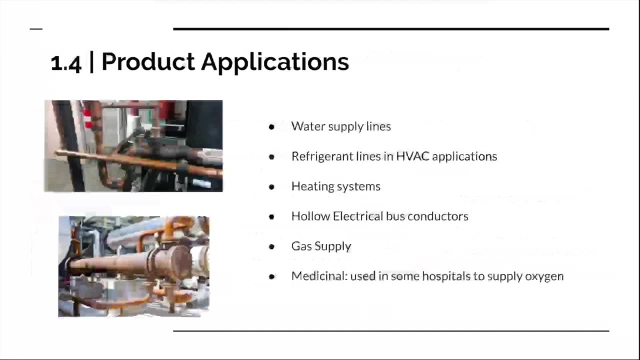 are located in moist, damp locations. The copper pipes are usually behind walls, etc. And they're usually going to be lightly ventilated, resulting in hot, extremely hot air. So if you have a hot or cold locations And finally, product applications, well, there are different ways that. 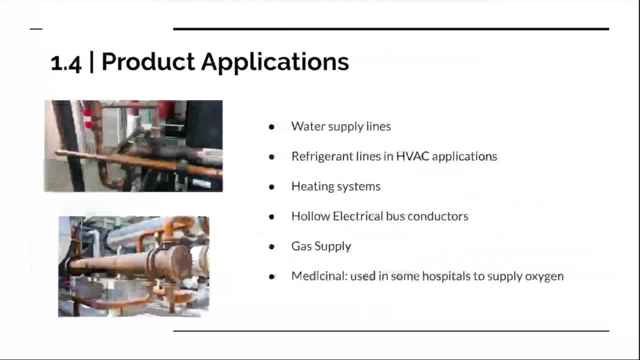 the copper pipes can be used. Here's a list of some of them, such as a water supply line, refrigerant lines in HVAC applications, heating systems, hollow electrical bus conductors, a gas appliance, and it is even used in some hospitals to supply oxygen and oxygen tanks. 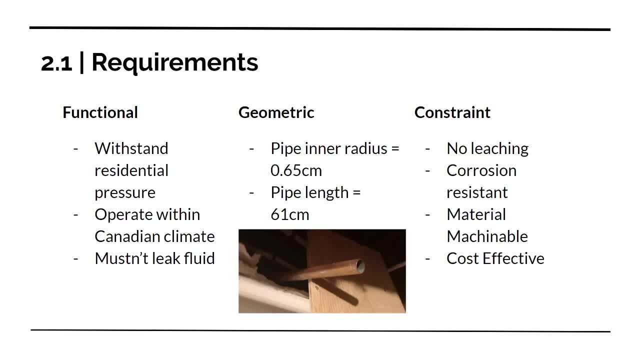 Now we can move on to our requirements. For functional requirements, we say that the pipe must withstand residential pressure, That it must operate within the Canadian climate and that it mustn't leak fluid. For the geometric requirements, we say that the pipe inner radius has to equal 0.65 centimeters. 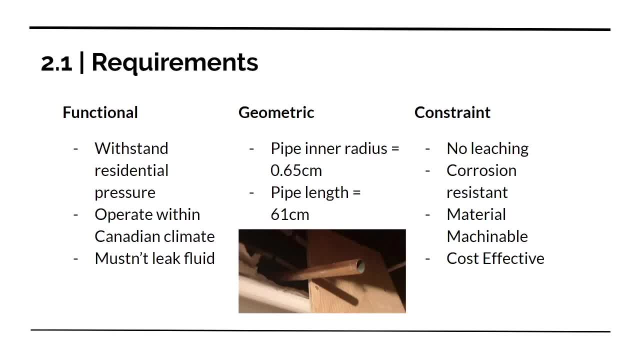 and that the pipe length has to equal 61 centimeters. These dimensions come from the original copper pipe. Lastly, for constraint requirements, we say that the pipe material must not leak into the water, that the pipe material is corrosion resistant, that it's machinable. 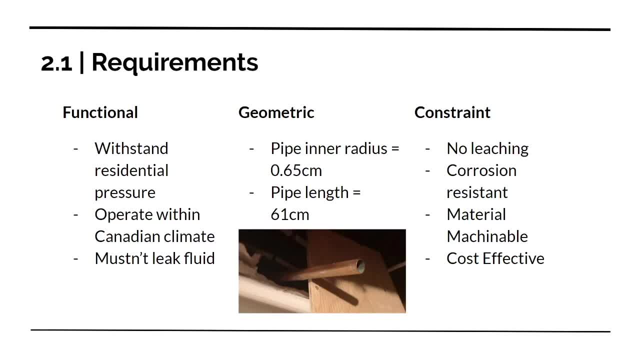 and that it's cost effective. When we say corrosion resistant here, we're specifically referring to resistance against failure. Leaching is also caused by the fact that the pipe is not shut by corrosion, so we want to make that distinction between the two, as they're important. 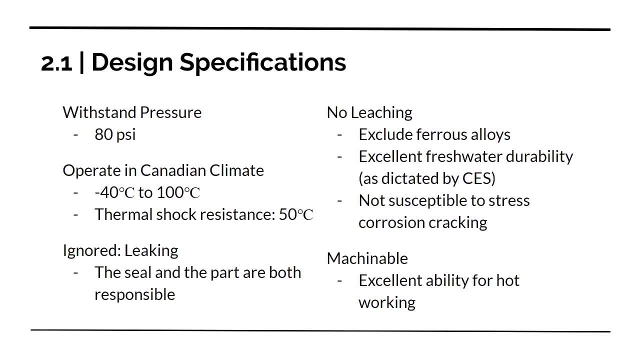 for different reasons. Now, to convert these functional requirements in to design specifications, we first find the residential home pressure and then say that the pipe must withstand it. We take extreme lows for Canadian climate up to the temperature of the fluid in the pipes and say that these, this is our range of operating temperatures. 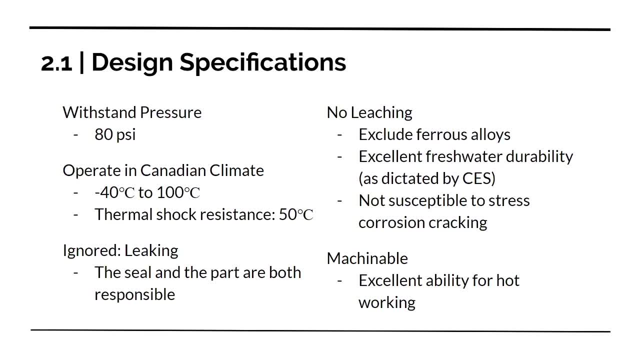 And we also include a thermal shock resistance clause of 50 degrees because we don't want the certain temperature to impact global agencies and I know that there are a risk factors around these. so just fired public power units and we must keep an eye on freak plug and other supply systems by all those known vessels to help us with making those modifications to comfort our total operation. and then back home, 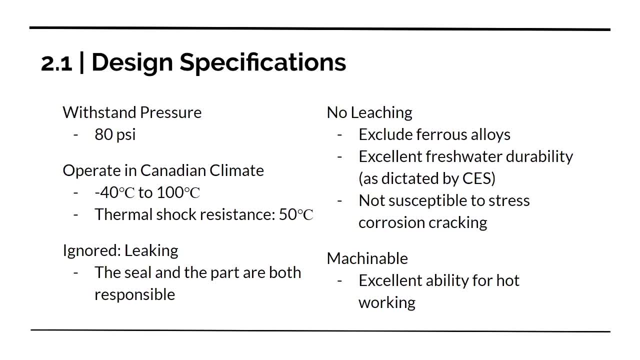 we don't want the part to suddenly fail due to fluctuation in temperature. We ignore the leaking requirement because leaking is a combined responsibility of both the part and the seal and it's hard to just rate a part based on the leaking. We use CS parameters in order to constrain our constraint requirements. 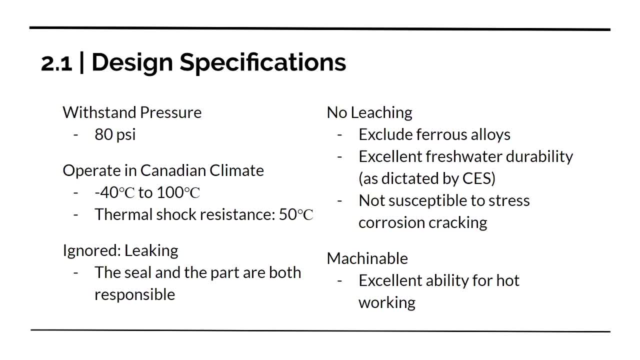 So we exclude ferrous alloys because we know them to corrode. We say that the fresh water durability must be excellent, according to CS, and that the material is not susceptible to stress corrosion cracking, so that it doesn't suddenly fail due to the material being in an environment. 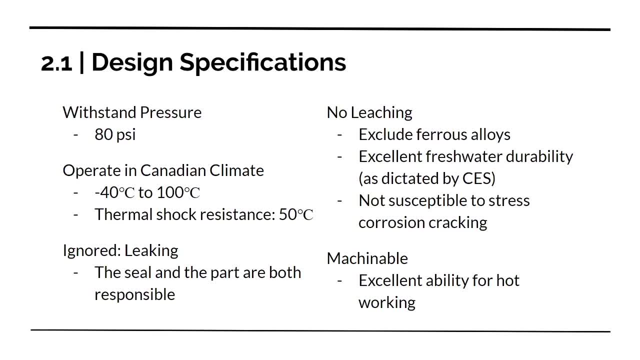 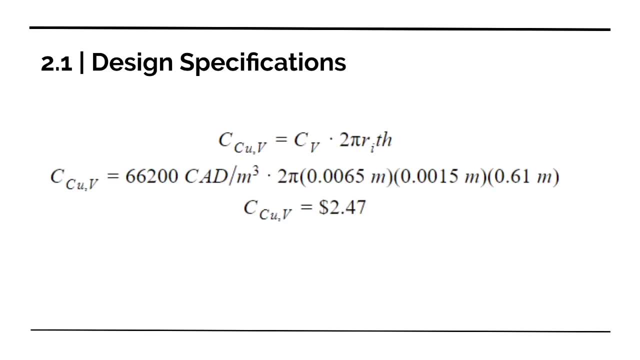 that's quite conducive to corrosion. Lastly, we say that the machinability must be rated at excellent. We do this cost analysis to constrain our cost. So what we did here was that we took the copper pipe, approximated its volume as a sheet rolled. 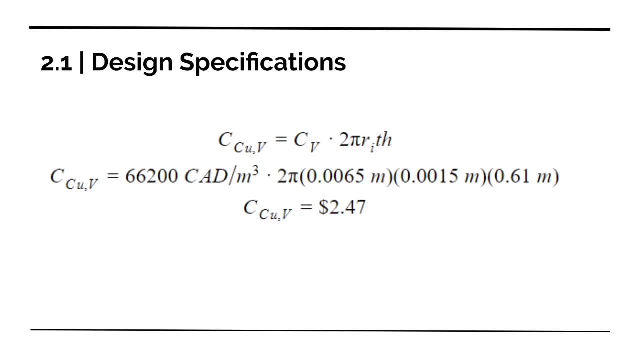 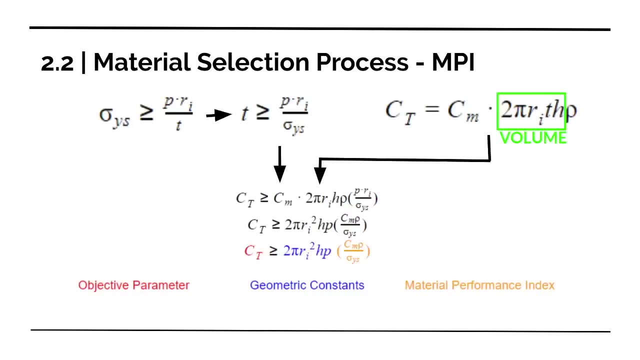 into The cylinder that we have. took the volume cost, multiplied it by that and found that the pipe would cost about 247 raw material. We then move on to our MPI. So first, with this equation, we relate the loading condition to material properties. We identify t as the free variable, as the thickness doesn't have a 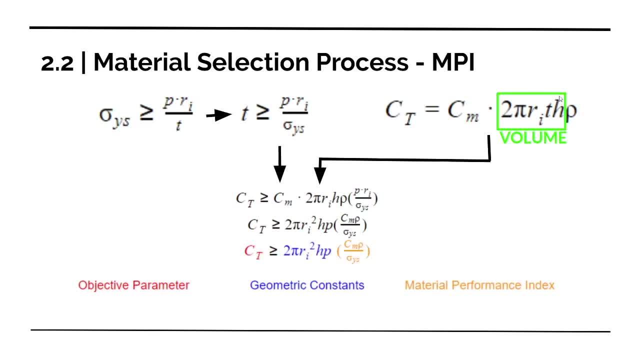 lot of bearing on the function of the part and then isolate for it here. Secondly, we approximate the volume equation for it- uh, the tube- using the same method that we did for the cost analysis. We multiply it by the density, then the mass cost, and that will equal our total. 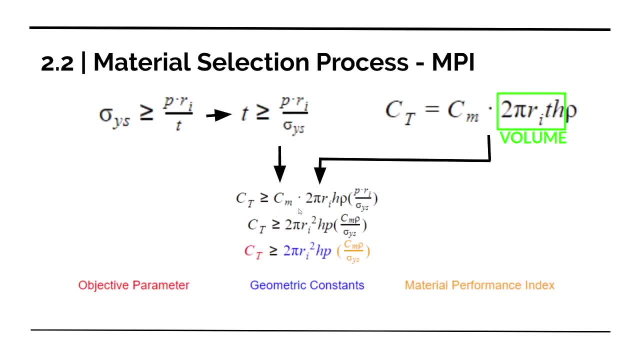 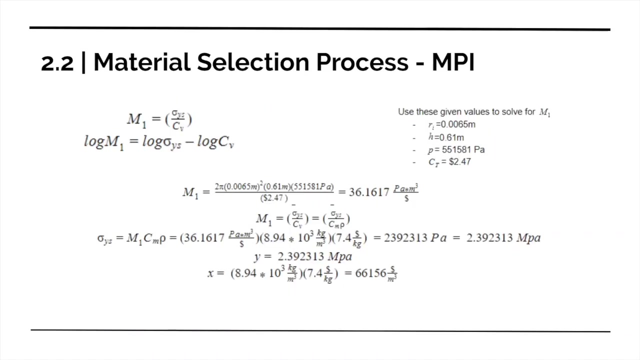 cost. This function has to be minimized as the cost total lowest possible value is defined by this function. So by minimizing it we reduce the lowest cost total value possible. To minimize this function we have to use the, this MPI, and say minimize it. First we inverted the MPI value so that we were looking to maximize it as opposed to minimize it. 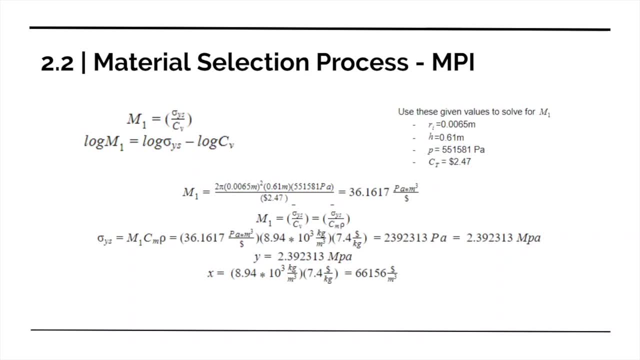 Secondly, we applied logarithms to this equation so that we could find the value of the slope for the CES graph. As the variables in this equation are all being raised to the power of one, the slope for the equation is one. Next, using various recorded and given values, we found this value of m1.. 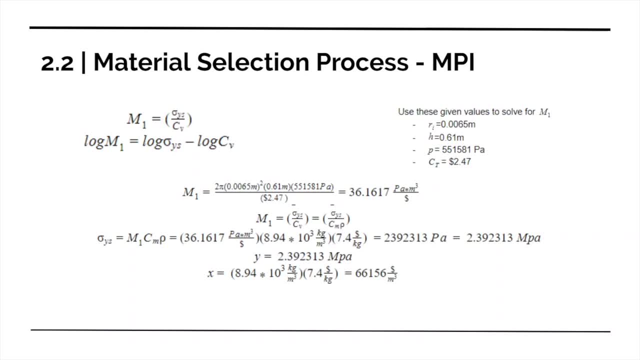 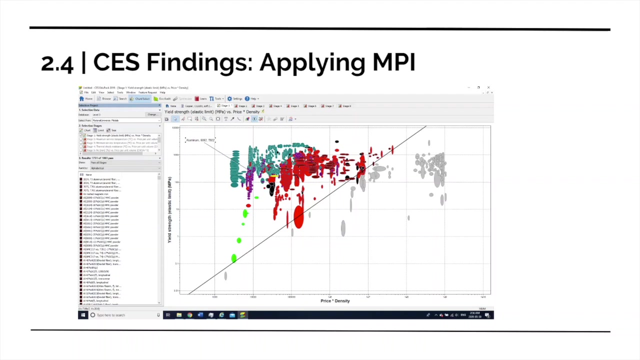 Using CES, we found the values of the density and the price per kilogram for the copper alloy of the component and, using m1 along with these, we found a point of on the line for the MPI. Applying this line to the CES graph, we were able to limit a decent number of materials and, as we're maximizing it, 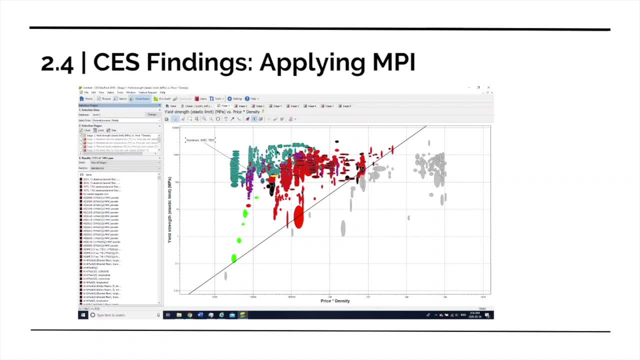 it is any value above the line that is acceptable. Next, for water safety and anti-corrosion, we had CES test for excellent fresh water performance, but the material was not susceptible to stress, corrosion, cracking and that there was less than five percent iron content in these materials. 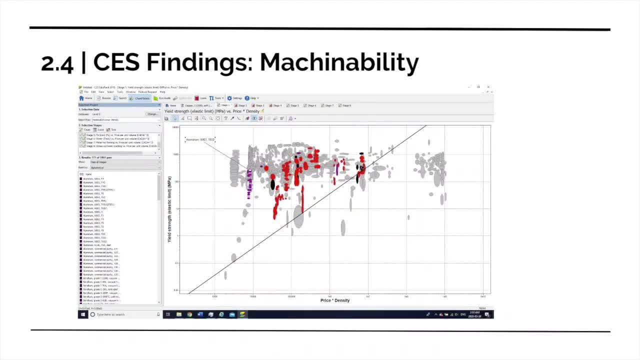 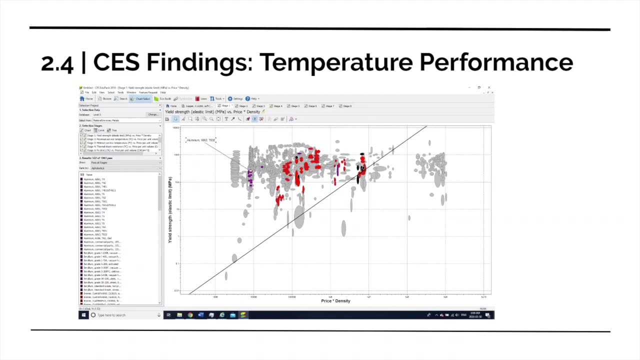 For machinability, we had CES limit to materials that had excellent hot forming. This is because the production for the pipe includes hot forming in its processes. Finally, for temperature performance: as the component is the inlet for a hot water healer, we made sure that the maximum performance temperature was at least 100 degrees Celsius. 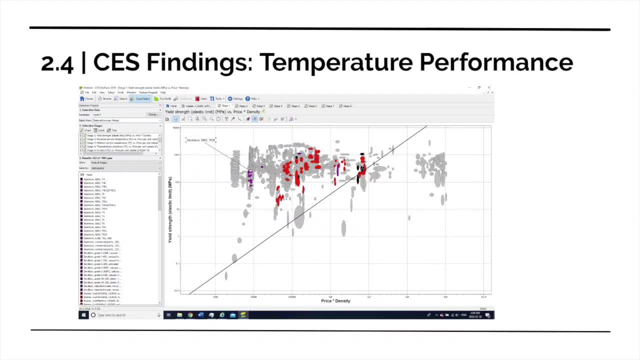 And since we are also living in Canada and we can endure harsh winters, we made sure that the minimum performance temperature was at most negative 40 degrees Celsius. Using a similar train of logic, since there might be great variations in the temperature of the water at the inlet pipe, we made sure that the thermal shock resistance of the material was also. 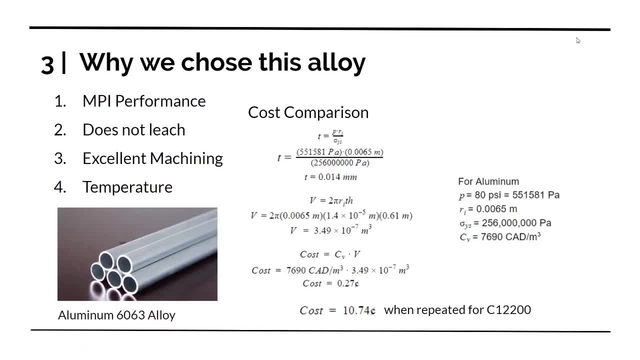 at least 50 degrees Celsius. Now we must explain why we chose this alloy. Based on the CES analysis, we know that all functional requirements are met. The material doesn't leach, it has excellent machining and performs well at all temperatures. We chose this particular alloy because it was second farthest from the MPI line. 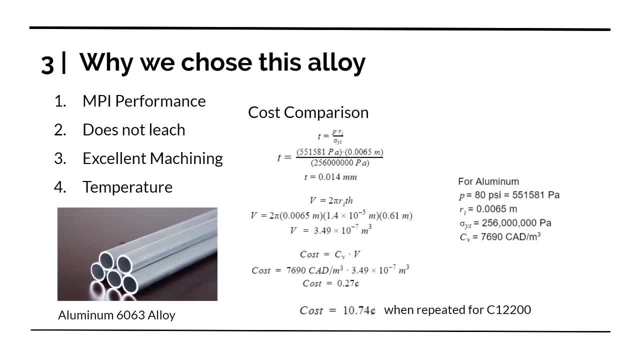 behind a magnesium alloy which is highly reactive and possibly dangerous for the home, so we disqualified it. To show the effect of this MPI in action, we do a cost comparison where we take the load condition and find the minimum thickness for the aluminum Based on that condition. we then find the volume based on that thickness. 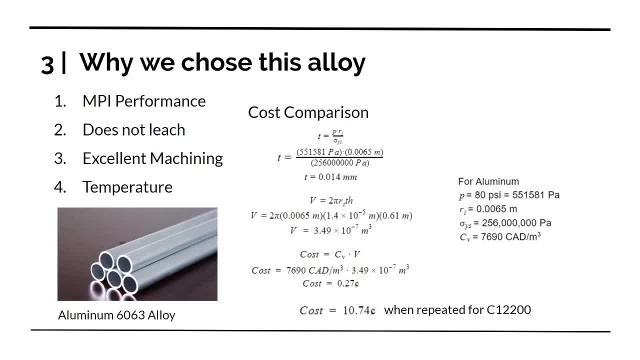 we take the volume cost for the aluminum and we find that per part it costs less than one cent. For comparison, we do the same for copper, where we find the minimum thickness, find volume, use the cost volume for copper and then find that it's 11 cents for copper raw material for. 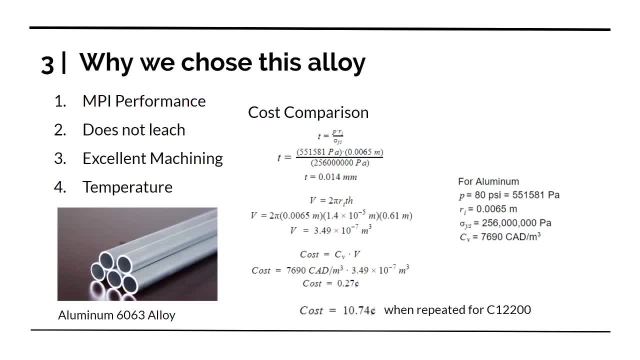 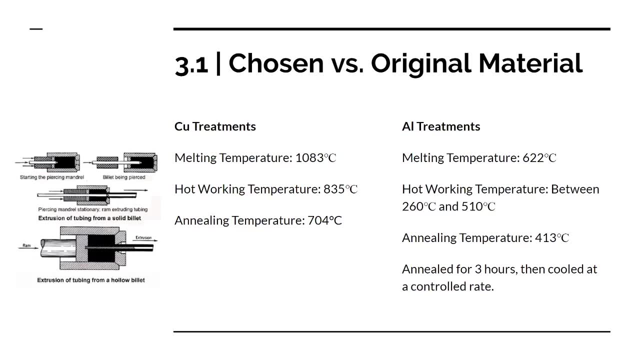 the same part, So two parts with identical performance. the aluminum is much cheaper. We reason that the machining is the same for both parts. so that means that machining costs won't vary too much and the difference in price for the part will be all in the raw material, which, you see, is quite a large gap. That being said there,